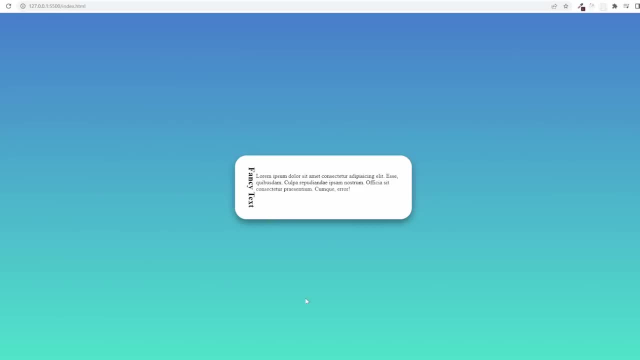 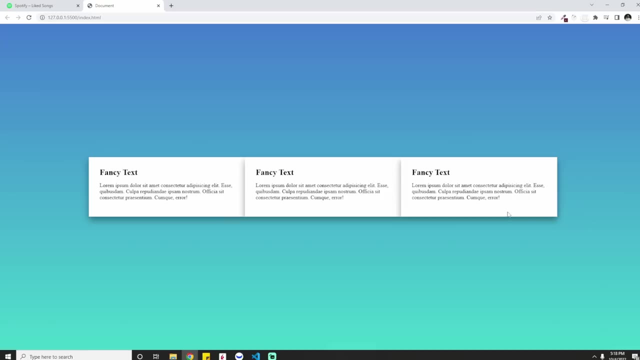 Hit save, Boom, Scale this up and automatically it looks fancy. Number two on the list is one of my favorites. actually, I haven't really seen it used as much as I wanted it to, but I'm going to show you And it's called gap. So if you're using flex and you're doing display flex in this case, 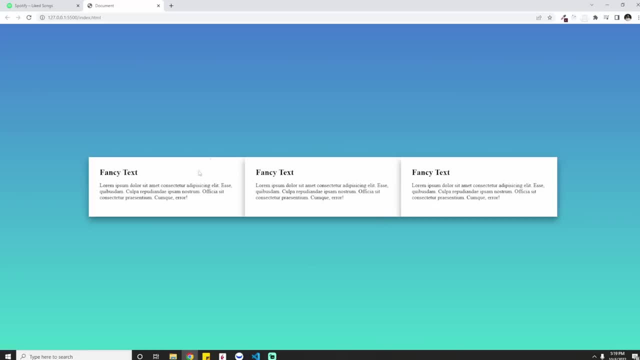 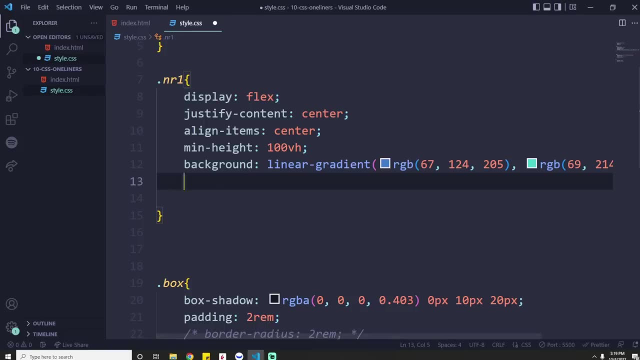 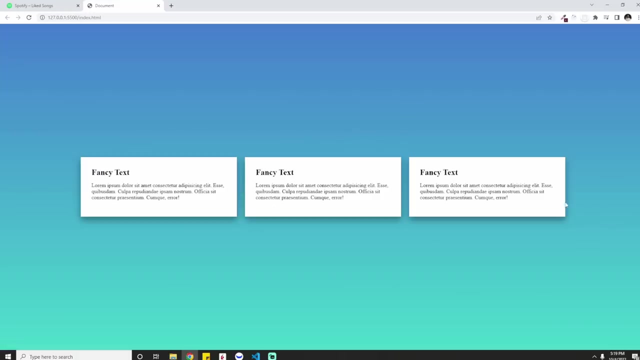 I just have a container here with three items, three boxes, and I want to add some spacing in between the items. All I need to do is not go to OBS but go here to my container. So I have display flex and just add the property gap And then I can specify a number of pixels, like 24.. And boom. 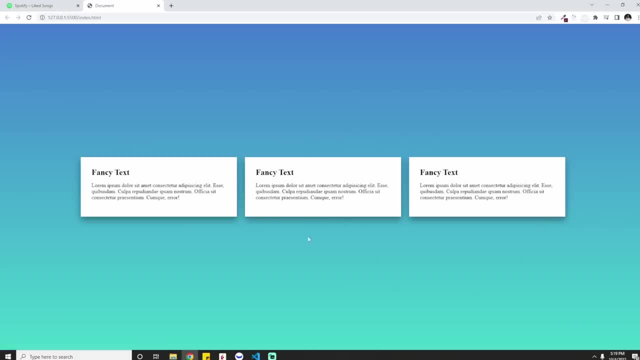 done, And you can also customize this to only be on columns or on row by adding column, row, column room, column gap or row gap, And that's it. Really simple one, but really useful, Okay, so go on and gap it up. 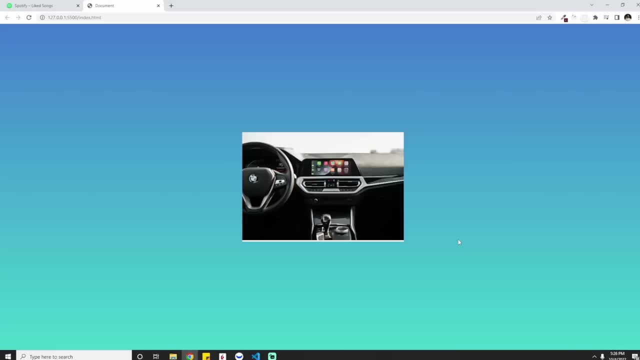 That sounds weird. Here's a cool little way that you can flip over an image either horizontally or vertically. So if you want somebody to point in another way, flip over a face. why would you want to flip over a face In this case? we have a car here, So if I want to flip, 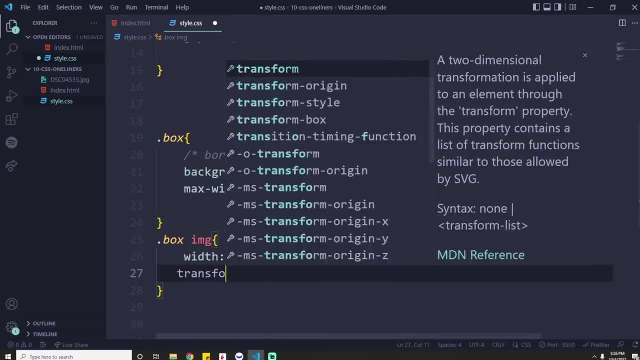 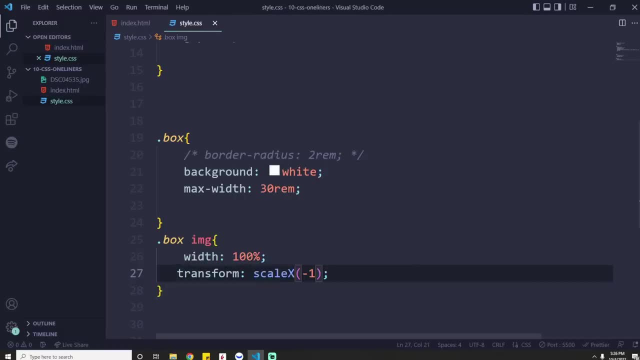 this over horizontally. all I need to do is the transform scale and do minus one, And I can do either X here or Y. So let's do X in this case And boom, you are in the UK. bitch, I love this one. 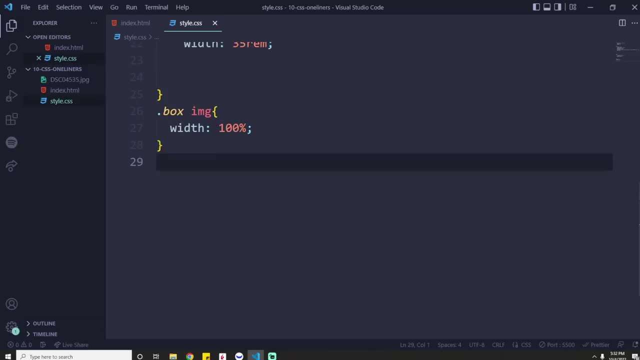 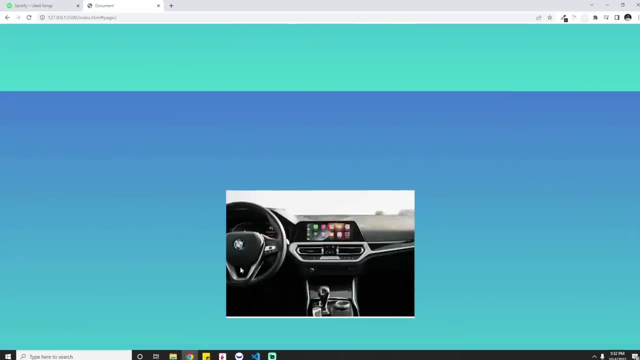 because it used to be so complicated back in the day, But now it's really, really simple. So let's say I have a page, two pages here, And when I click on an anchor tag I want to smoothly scroll down to this one, But, as you can see, the default behavior- it just automatically jumps down like 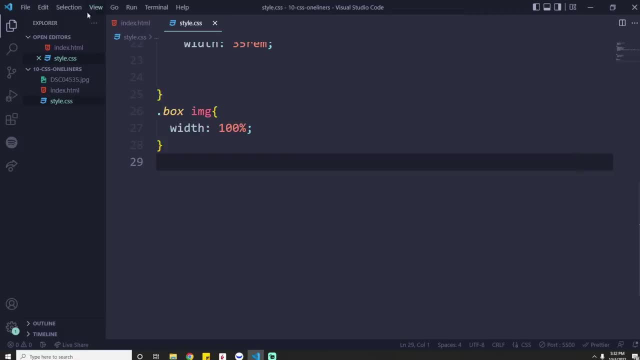 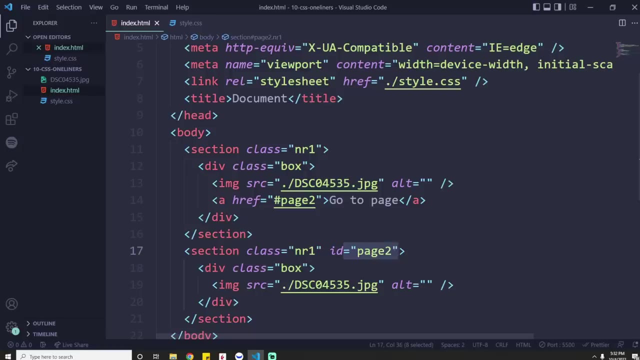 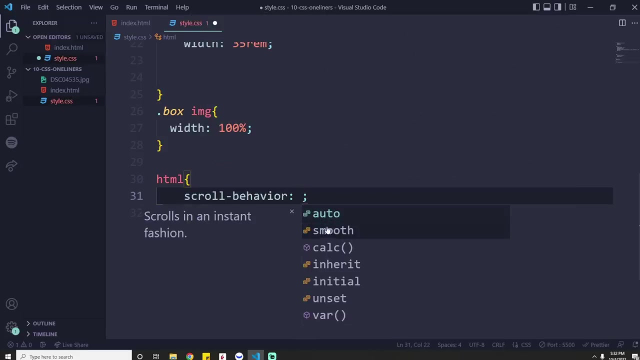 that Oof. So to add a smooth behavior, all you need to do is you need to have your anchor set up here, right, So it takes us to page two. It has an ID of page two, And then just grab your HTML and say: scroll behavior, smooth Like that. And that's it, It's. 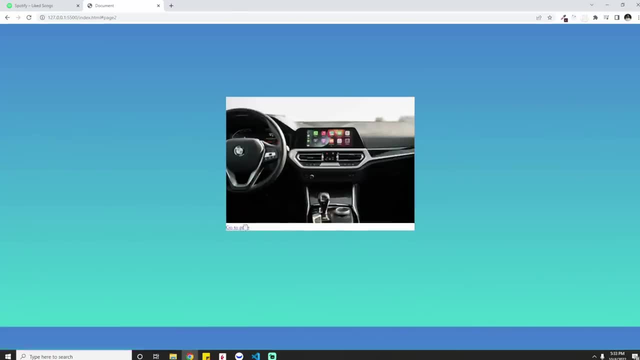 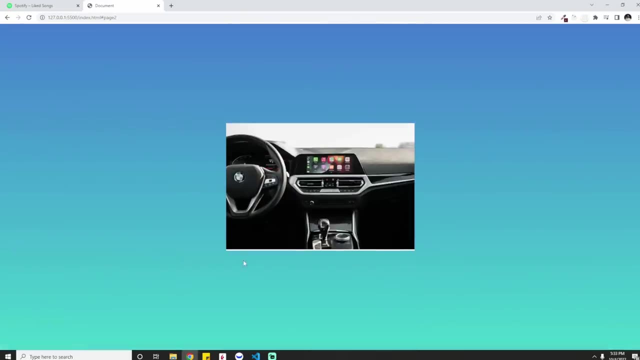 safe. Take a look, That is crazy. That is absolutely crazy. Look at that. One line of CSS and you have a nice, smooth animation going. This is a really, really cool one. If you want to make Airbnb type cards, Excel type snap cards, Now you can browse each listing on Airbnb like that. Well, in our case, 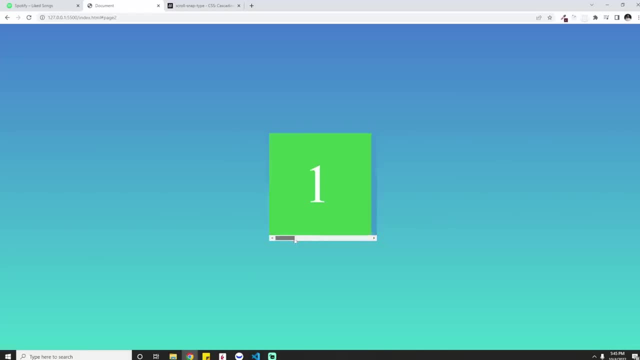 I have it: one, two, three, four, five, And we're going to look through the code so you understand this a bit better. But if I go here and stop, nothing happens. So what I want to do is, when I scroll like that, it should snap to that and then snap to that, and snap to that. So what is? 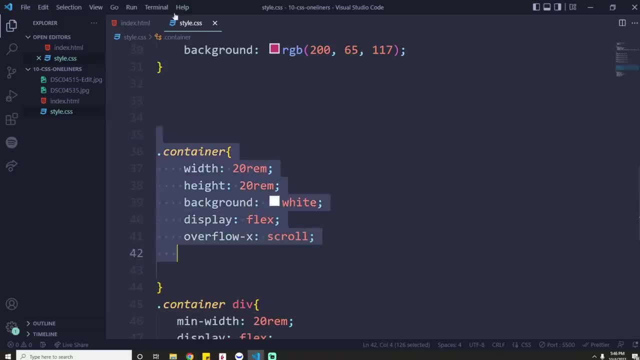 this. How is this code set up? And then I'll show you kind of what we have. We have a container here and just a bunch of divs inside. Okay, So, container with a bunch of divs, And all I did was I set the height and the width to them and add a display flex with an 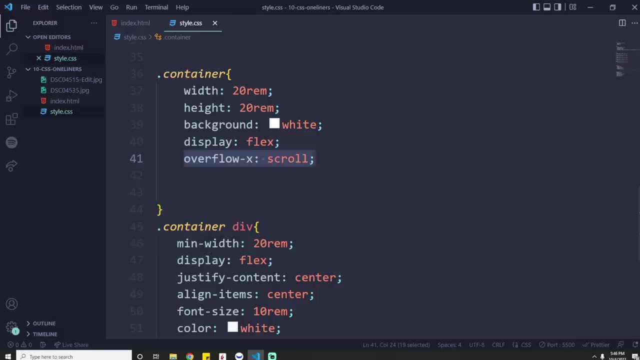 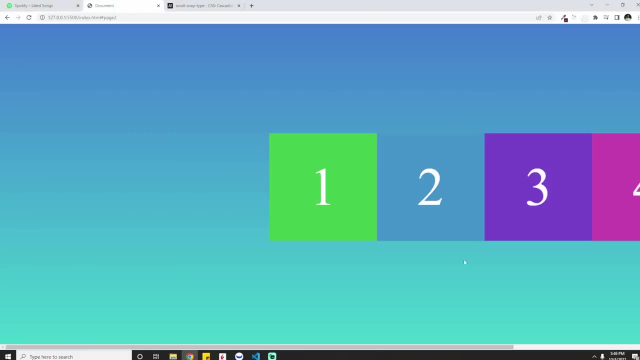 overflow X of scroll. Okay, So we can scroll And then the min height on the divs take up basically the same height as this. All right, So if I don't have this overflow X on it, you're going to see that all the content overflows like that. But with this one we got the nice scroll bar. 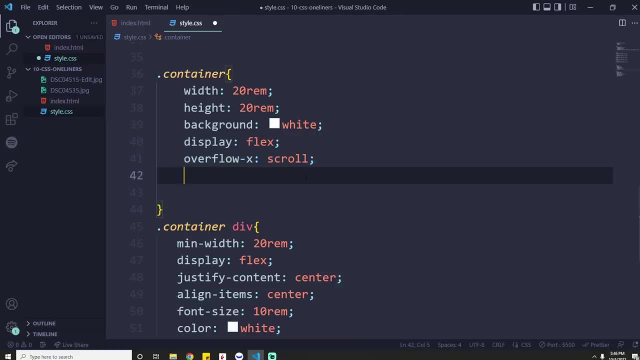 Scroll bar. So how do we add this thing? So all you need to do is it's two properties, but it's really short. Scroll scroll- snap a line. I cannot speak anymore. Scroll scroll- scroll- snap a line. 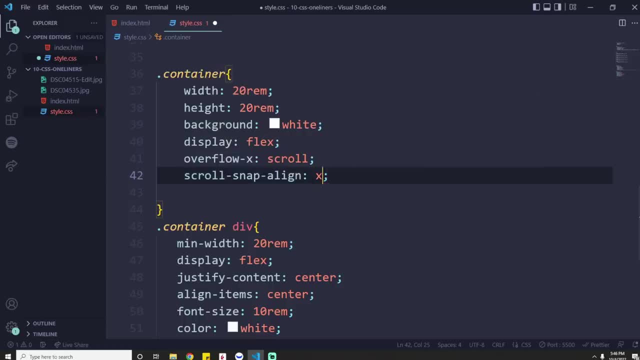 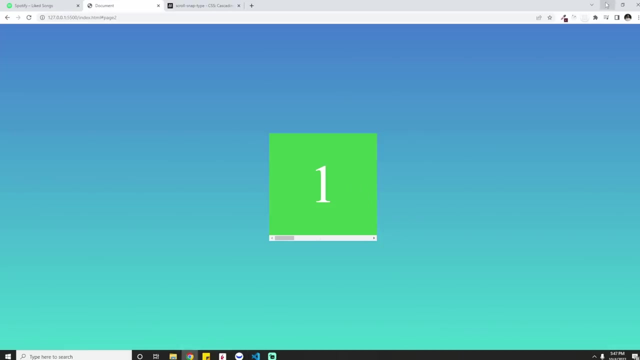 and we'll do X and we'll say mandatory, Mandatory, Okay, So you can do it. Y as well. If you want to make like a- you know, like you scroll up and down and then it snaps to the page- you can do that as well. So that's one, And then to each individual item you have to tell it. 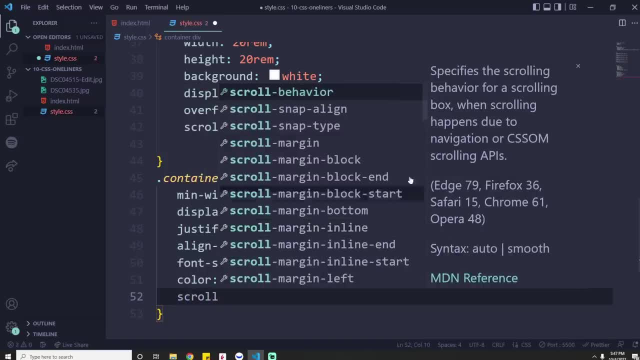 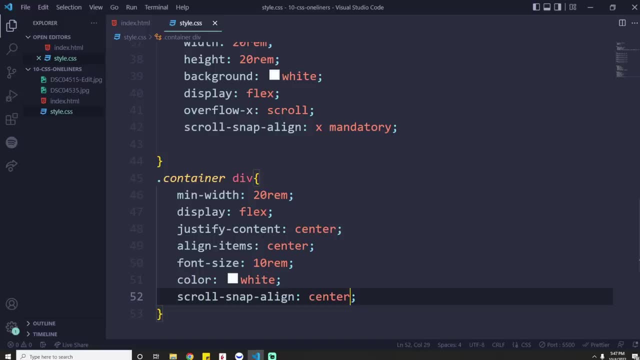 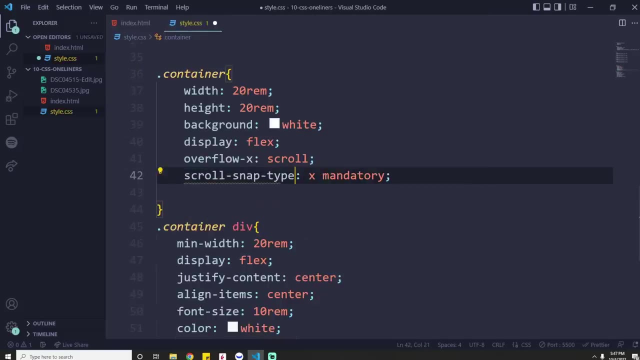 basically where it wants to snap to, So scroll, snap a line and we basically want it to center. So now when we go like that it's not working, What's not working, X mandatory, Not a line here, Type My apologies, Scroll, snap, type, So X mandatory, And look at that When I 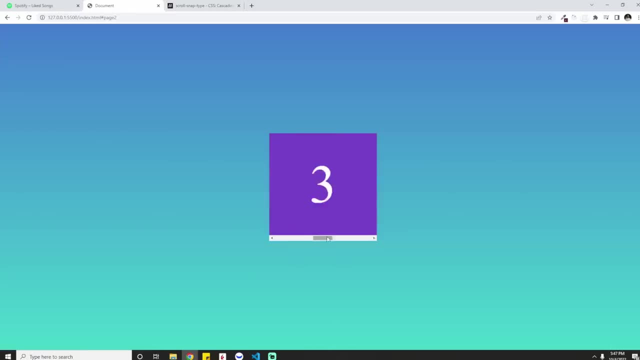 stop, it snaps to it. Now here's the cool thing about this: is you have a bit more control over it. You can also define some of the things that you want to do. So, for example, if I want to do a something called proximity and this basically lets you see it doesn't snap to it. You can kind 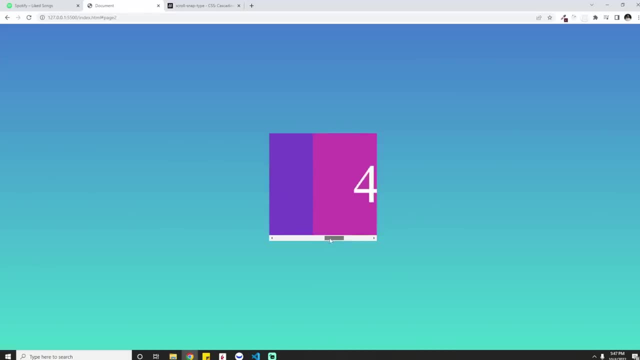 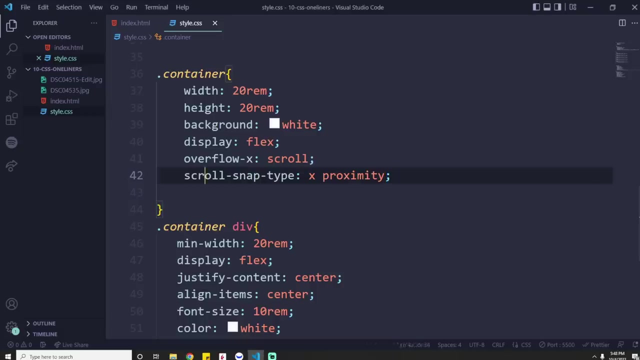 of move around freely, but if it's really close to the edge, only then it snaps. So that's, yeah, you can kind of play around with this. It's quite cool. This gives like a more natural scrolling experience, to be honest, But yeah, really like it. Really cool little property that you can use. 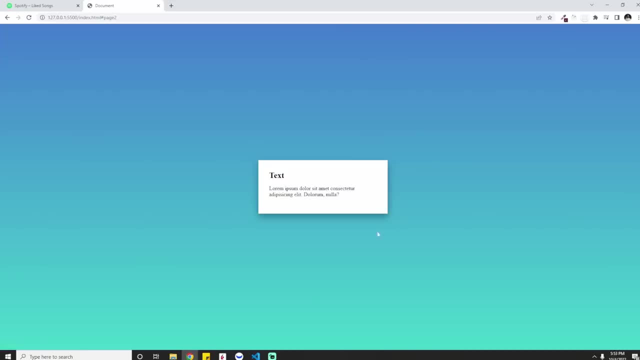 Scroll snap type. Okay, I absolutely love this one. Do you know how, when you have a text area, you can just grab the point here and resize it to whatever size you want? Well, you can do that to any element you want by using resize both. So go to your code, go here to box. All you need to do. 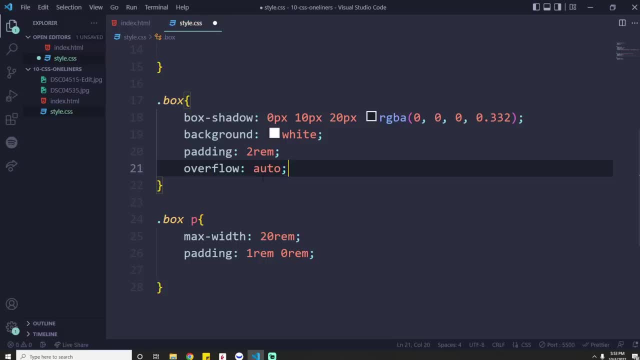 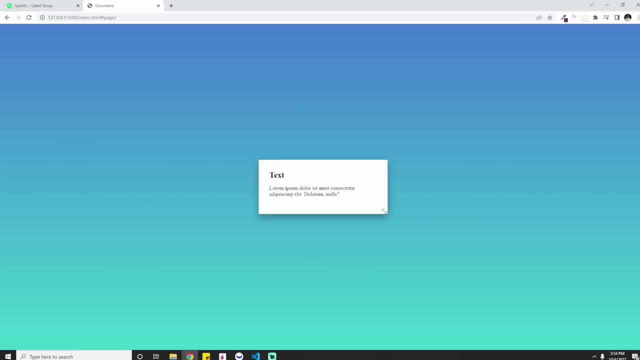 is: add a overflow of auto, And then all you need to do is say resize and say both And that's it. Take a look Now I can grab the end of this and absolutely resize it to whatever size I want. It's always going to keep centric because I have a display. 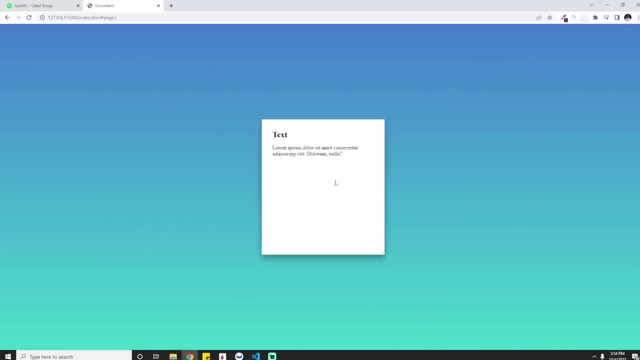 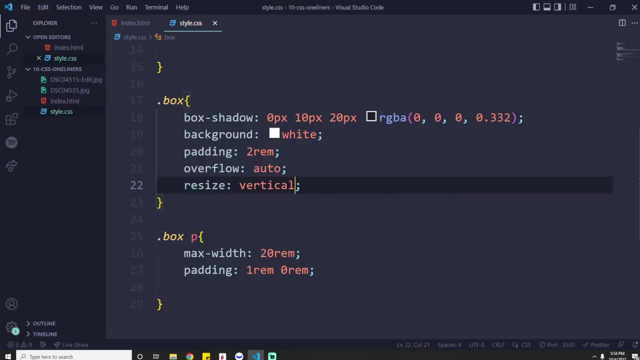 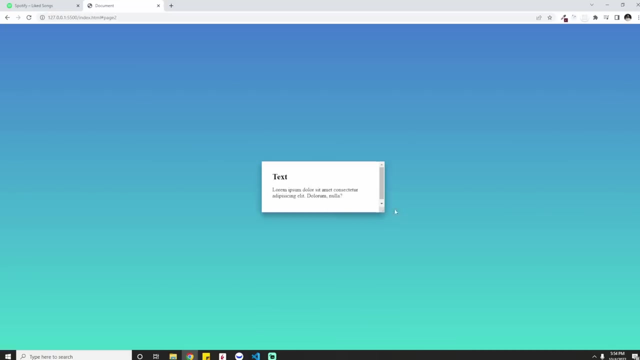 You can see the effects on it. Well, look at that, It's pretty cool. If you want to constrain it to only one axis, you can do resize. I think it's vertical, Yeah, And then also horizontal as well. And look at that: Boom, boom, boom, boom, boom. Okay, That's that. That's just a fun one. 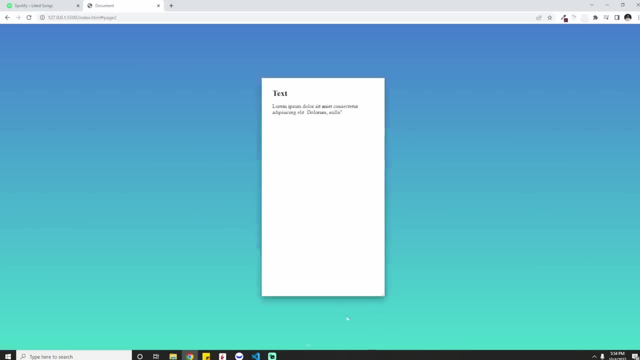 really Good luck finding something useful with this one. Here's a cool little trick to cut your text off. So if you have loads here and you don't want all of it to show up, you can truncate it. You're going to see articles use this a lot where only kind of a preview shows up. So the way you 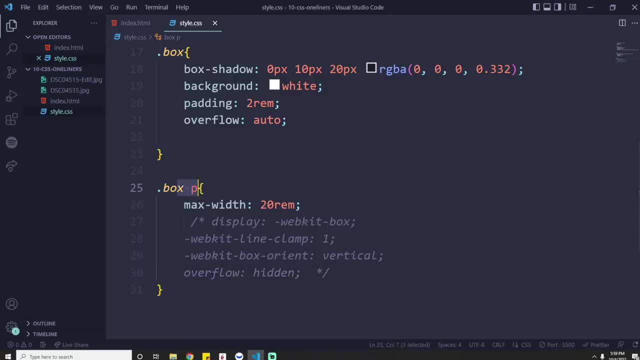 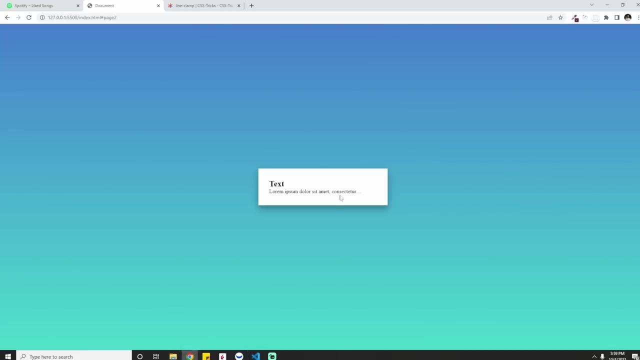 can achieve that in CSS is: just grab your paragraph from your box, add a display of webkit box to it like that, And then you can specify how many lines you want to show using line clamp. So if I do one, it's only going to do one. It's also going to add the dot dot dot at the end there. 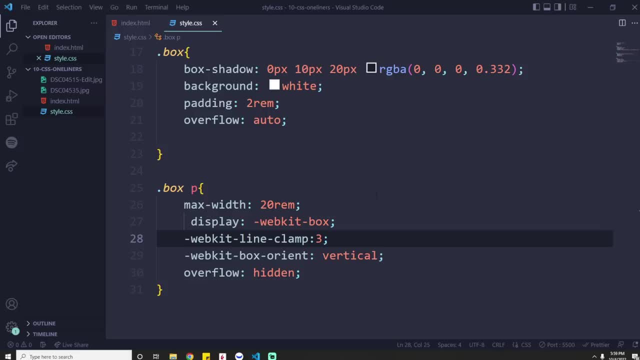 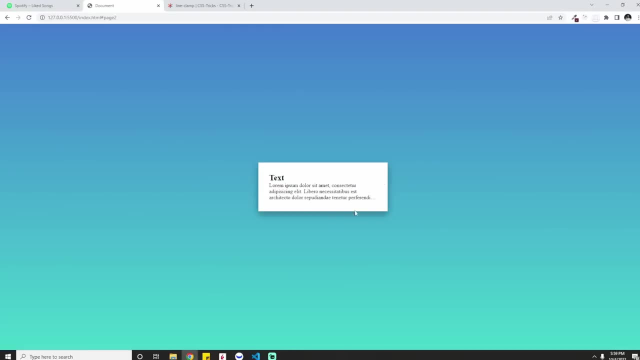 which is really cool. So let's say, in this case, I want three, Boom, easy peasy. And then you add the orientation, that's all vertical, and then overflow, hidden, Because if you don't do that, then you can just see everything and scroll won't work as well. So 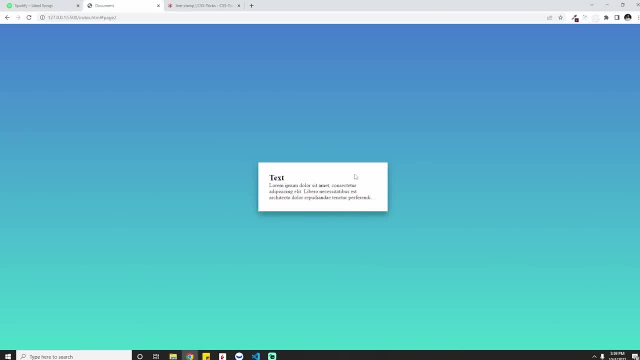 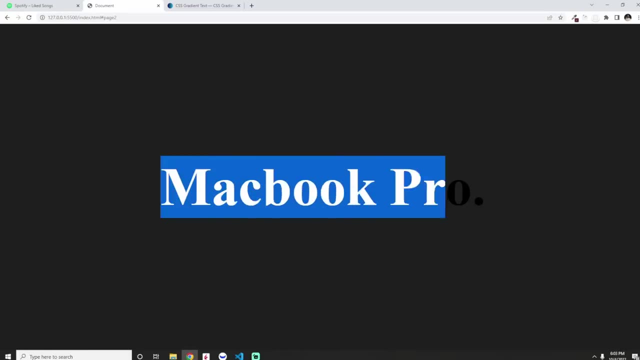 make sure you do over overflow of hidden, And that's that really simple but really effective. Let's say, I have one of those fancy MacBook websites and I want to add a linear gradient to our text here. Well, how can we do that? Well, if you go and add a background color to it. 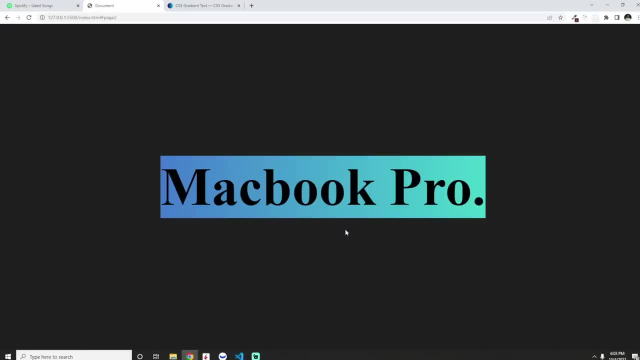 or if you try a color of gradient, it's not going to work. If you add a gradient, not going to work. If you add it to the background, it works on the background, But the way we can solve this issue is add it to the background. 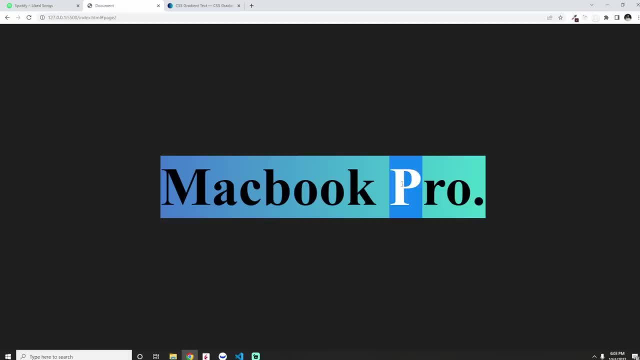 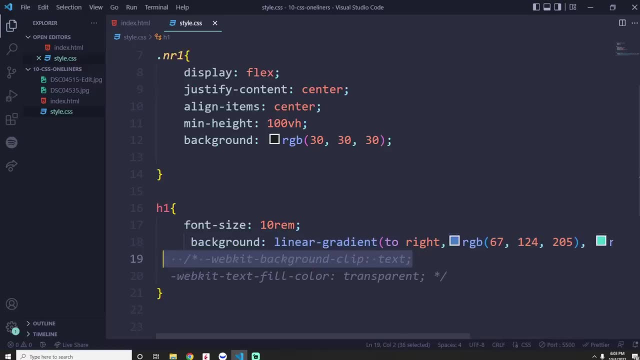 And then we make the text transparent and we'll basically mask it to the text. All right, So what we can do is add this property here of webkit background clip text, So that, basically, if I remove this comment, there we go. I'll still keep this. 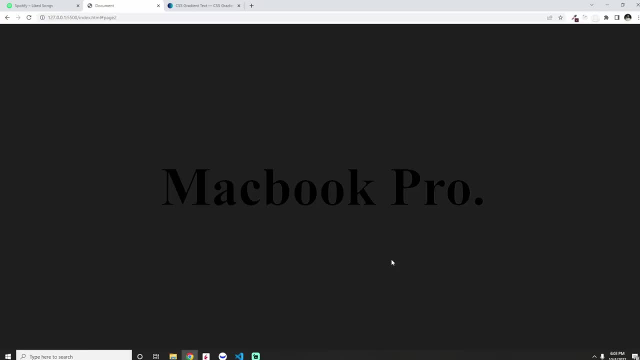 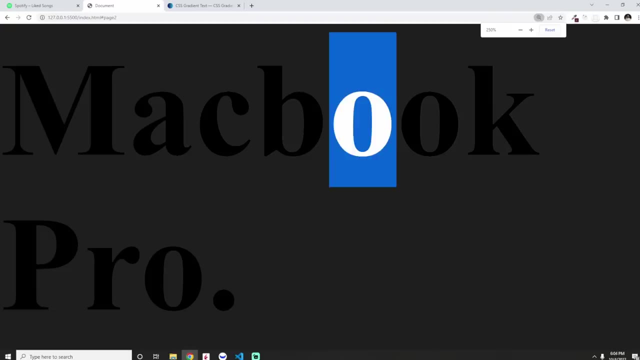 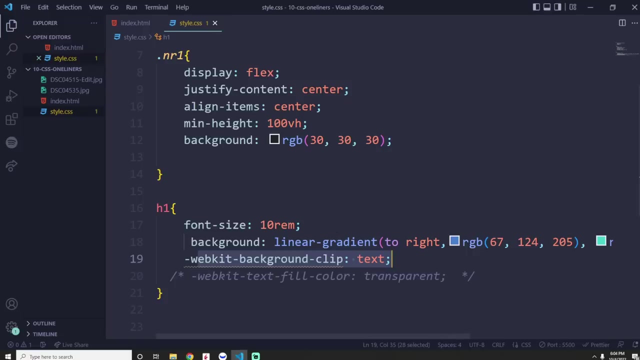 I'll comment it out. You're not going to see what this does, but essentially you can actually kind of see it. See, eclipse, that gradient to the text. So behind this black text is that gradient now, But what we want to do is make this text in the front transparent. So that's exactly what we do. 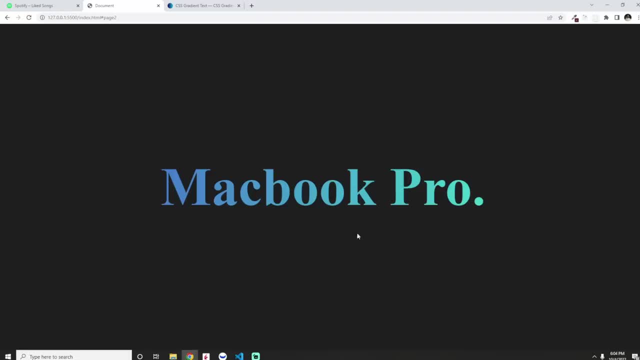 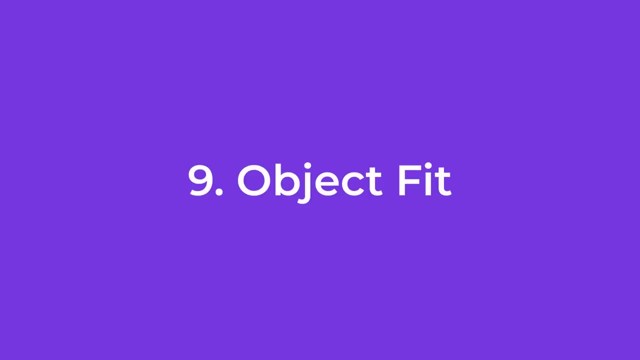 in this next line Text fill color. We'll do transparent and get rid of that black. And now the background pops true And we have this nice linear gradient. This is a problem I see loads of people having and the solution is so, so simple. So let's say we 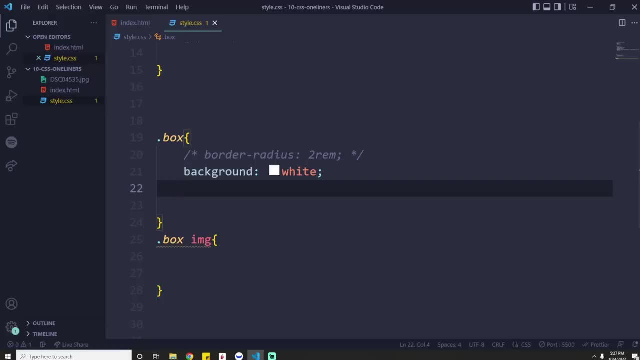 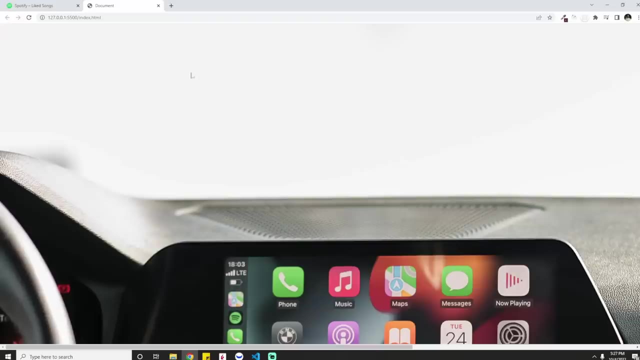 have a case where, again, we have a box and just an image inside and no heights or widths are specified. So by default, that image is going to go loco. As you can see, it stretches all the way out. It doesn't care where the box is and that's it. So what you do normally is you add a width of 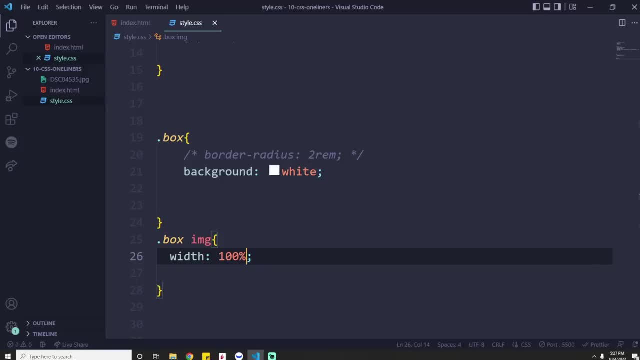 100% to this and then okay, so that's scaled properly, but it's going to scale according to the size of the box. So if it's not Specified, it's still going to take up all the space. So we can add a width and specify a width. 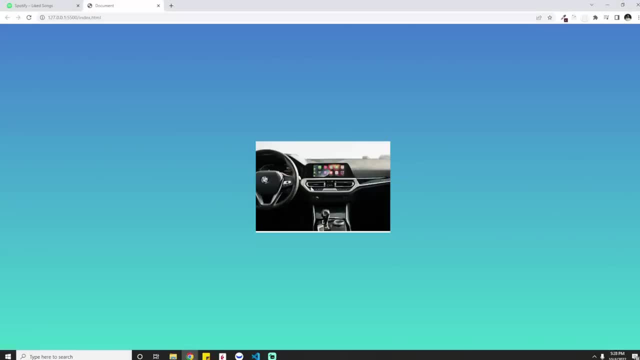 of like 25 rem to it. So boom, Okay, That's fine, That works All right. It literally fits to the box's size. The problem here is what, if I want to maybe have the box a bit more vertical, so I can do? 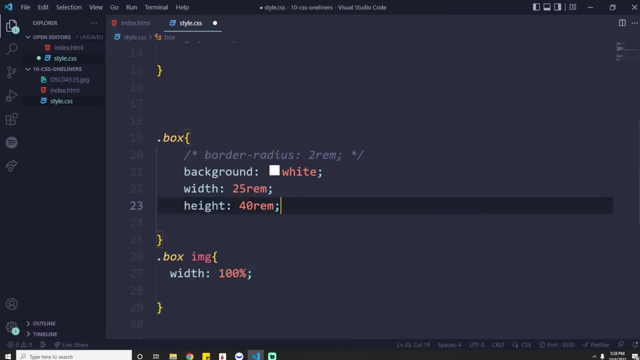 something like height 25,. let's do 40 rem, All right, Kind of like an Instagram type post. All right, I don't want this. I want this to kind of fill it all the way up. So yeah, you do the same. 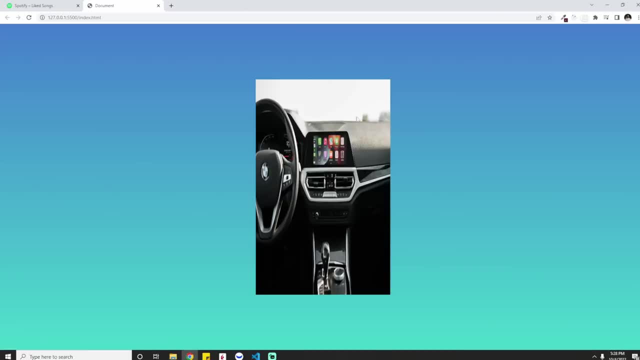 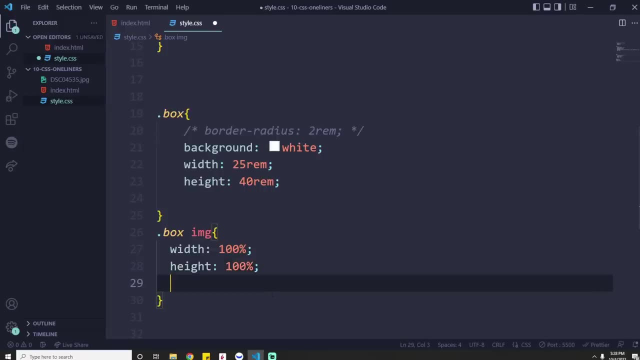 thing here. You do height 100%, So it fills it up. But here's the problem I want to get to. You have this weird stretching effect. So if you ever encountered this weird stretching effect, all you need is this object fit property And I think by default it's contained. But if you want, 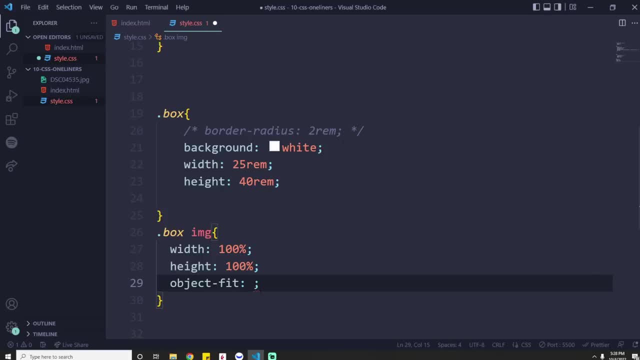 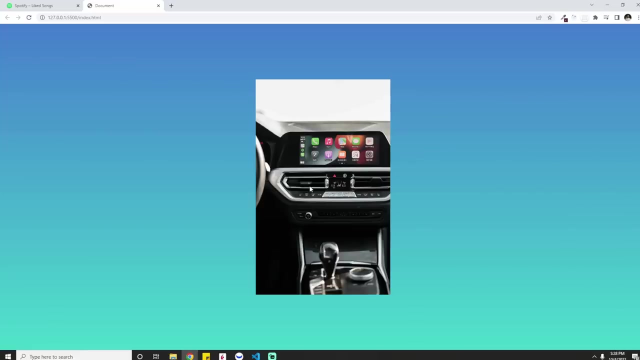 to get rid of this stretching aspect ratio problem, all you need to do is say fill, not fill, sorry cover. There we go, That's the one And boom, Because it actually zooms in on the image and it stops the distortion from happening. 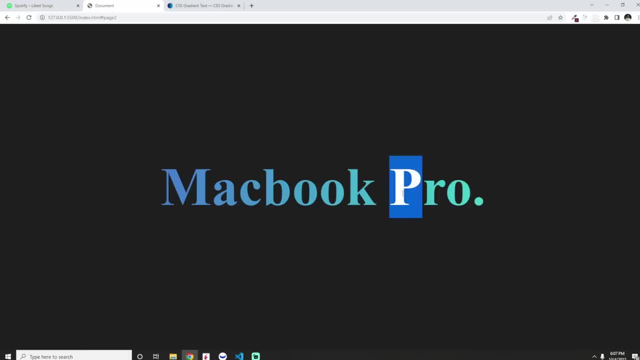 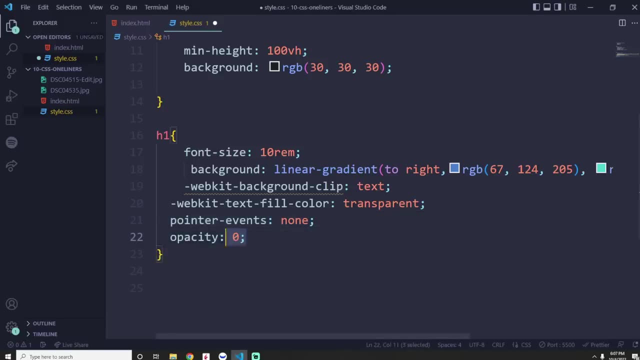 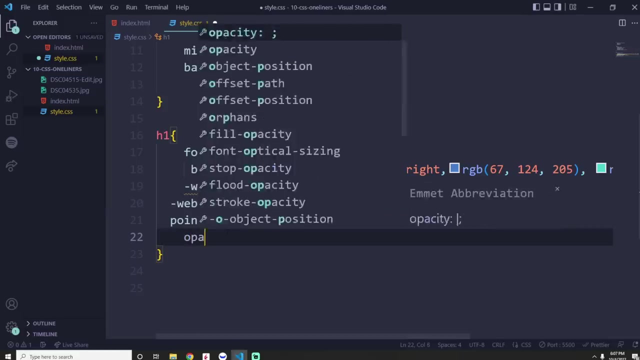 The last I want to cover is something very, very useful. It's called pointer events. And what pointer events does? it basically stops us from selecting an item, any item. So we can add pointer events, none, And now I cannot select this item anymore. Now, this in combination with opacity- 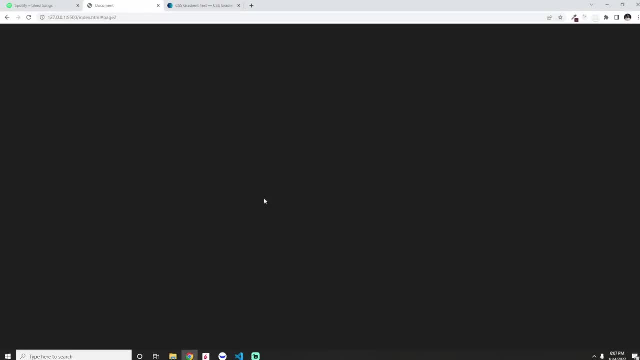 zero is really strong because we can animate this text popping in And, as you can see, I cannot select it. If I don't have this pointer events, none on it. I can still, if I know where the text is, see how the cursor changes And depending on what type of elements you have. if you have an image, 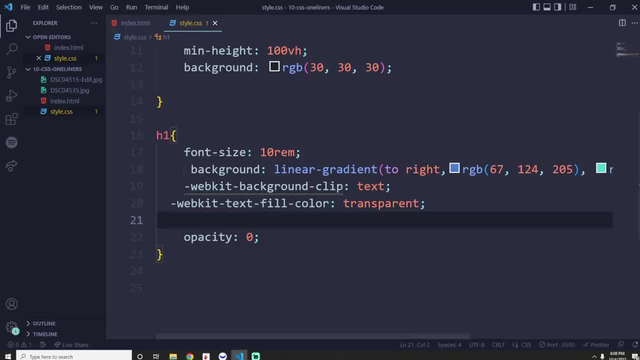 you can actually grab it, But yeah. So why do we use this rather than just doing something like display none, Because that actually gets rid of it completely. The thing, though, here is when it comes to animation. So if I want to animate this in on display none, it's not going to work. 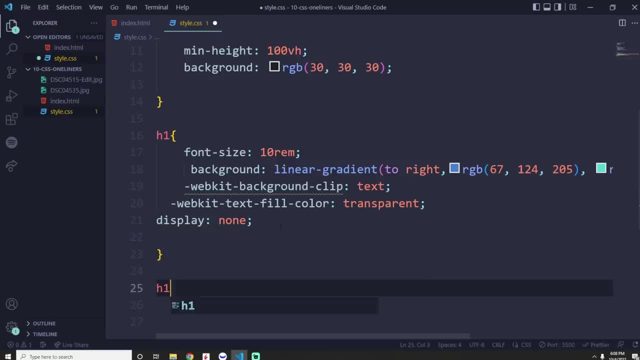 So I'll just add like a hover to this- Well, you cannot even do hover on it, but let's just add an animation in here. I'll do a quick key frame, So key frames, and then we'll call this fade.